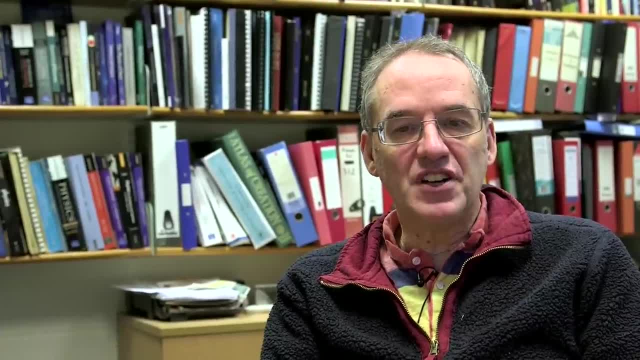 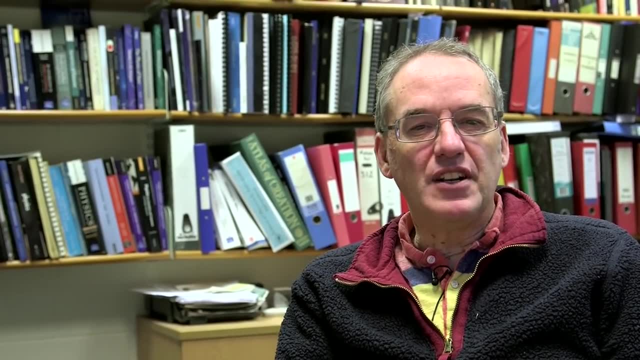 It does seem fairly obvious. It's a kind of a formal way of saying: really there is only one definition of temperature and that there is no way you can actually come up with a system where temperature is defined in a funny way such that one of these bodies has some 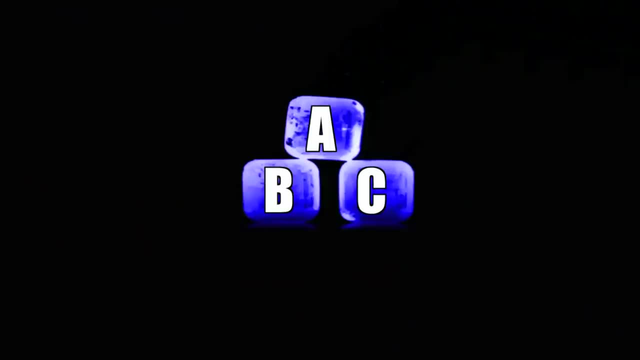 peculiar property, such that its temperature as far as body A is concerned is one thing, but its temperature as far as body C is concerned is another thing. And I think, because it is sort of stating the obvious, I think it's a good thing. 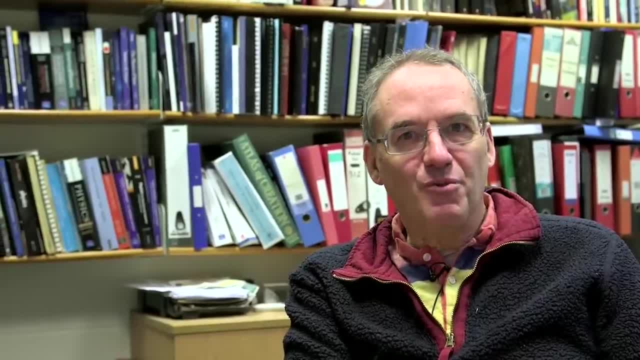 So I think that's why it's the zeroth law. So the first law is also fairly obvious in that it's basically a sort of restatement of the conservation of energy In thermodynamics. there's kind of two sorts of energy There's. 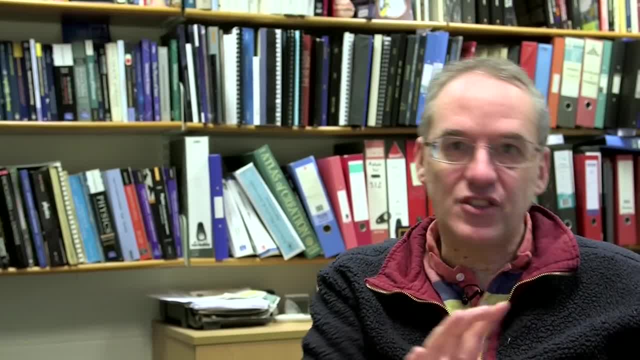 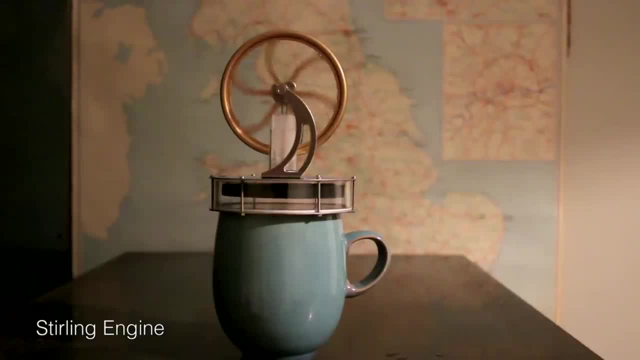 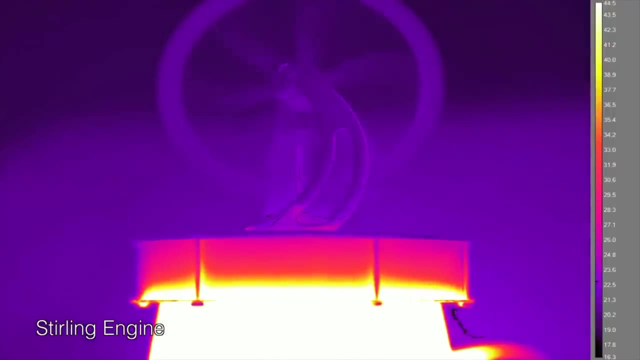 useful energy, which is work. So that's when you, if you push something or whatever, that's sort of applying energy to it and that's useful energy. And then there's useless energy, which is heat, And what the first law says is that it's useful energy which is heat And what the first 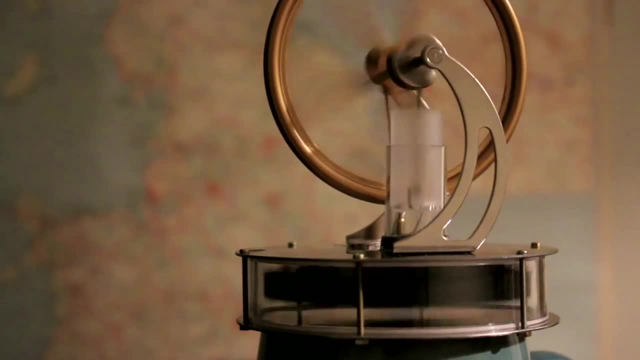 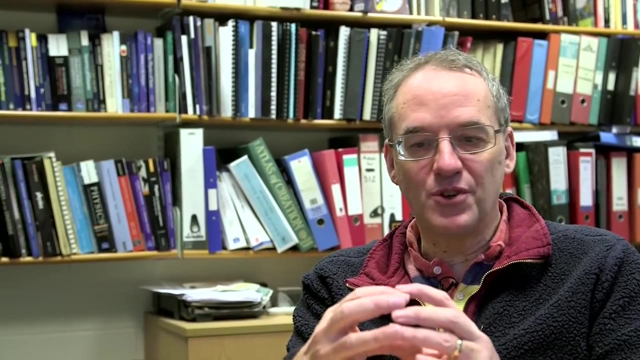 law says is that if you've got a body and you apply a certain amount of work to it- so that's one sort of energy- and then you add a certain amount of heat to it, the total energy of that body will be whatever it was to start with, plus the energy you added from. 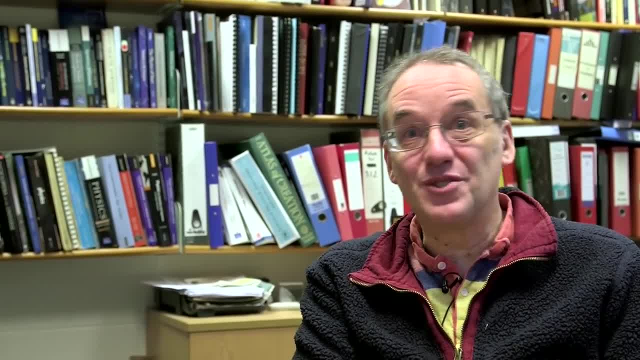 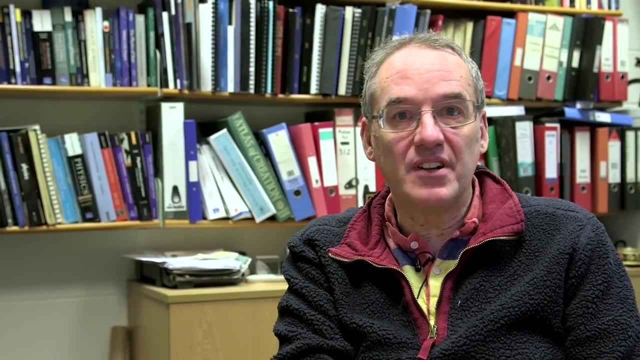 the work plus the energy you added from the heat. So it's really just a statement of the conservation of energy really. So I mean, there are kind of obvious laws, but you have to start with the basic building blocks in order to build up the entire subject of thermodynamics. And these are really the 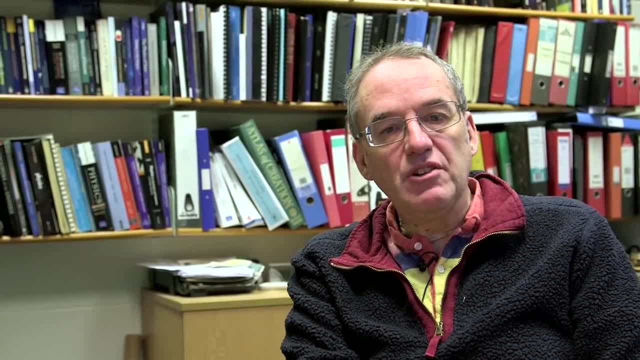 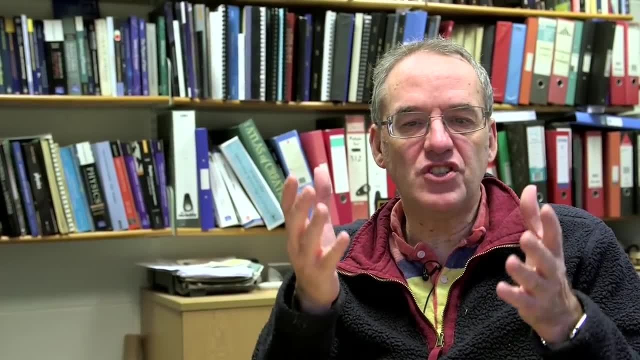 most fundamental building blocks. The third is difficult to talk about until we introduce the concept of a thing called entropy, which is to do with the disorder of a system, and the third law is basically saying that as you cool a system down towards absolute zero- the degree of disorder, so this quantity, entropy, drops towards zero, or at least 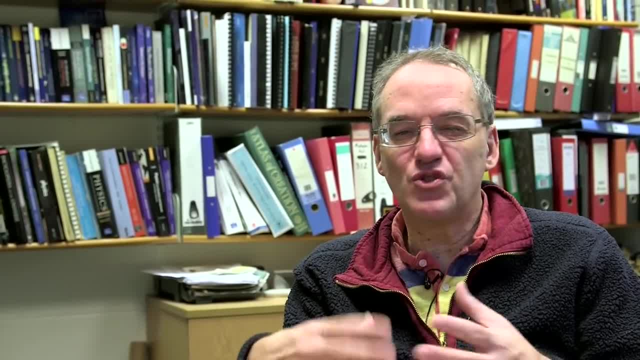 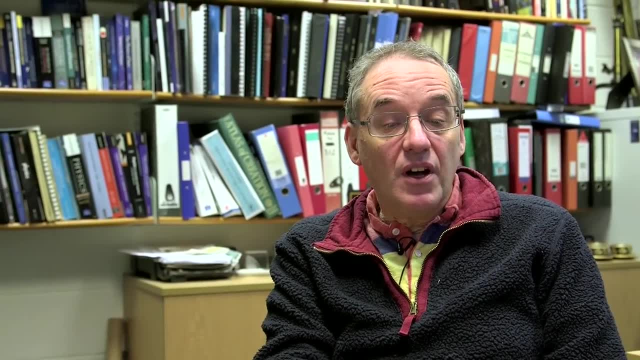 drops to a very low value, so classically it will drop to zero. there are some sorts of systems: it'll just drop to a low value but it will decrease until you get to absolute zero and then it will stop. so the second law has has various formulations. the first formulations were put together really before this idea of 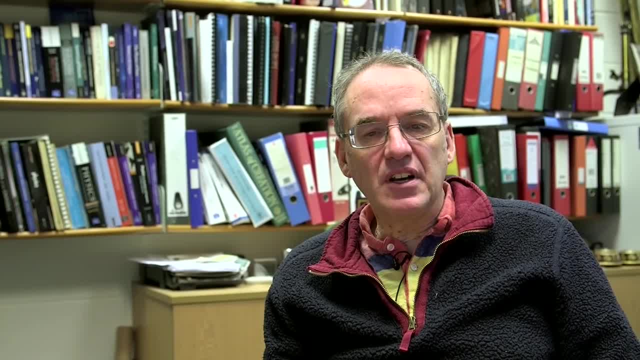 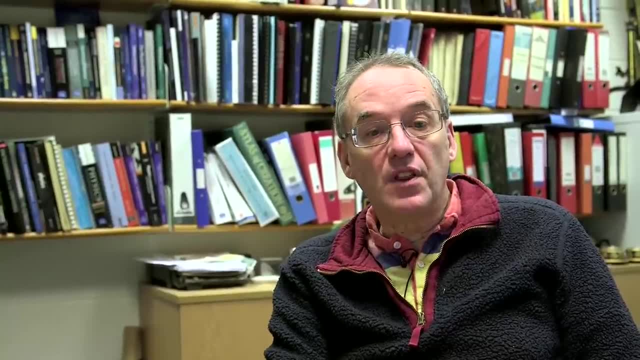 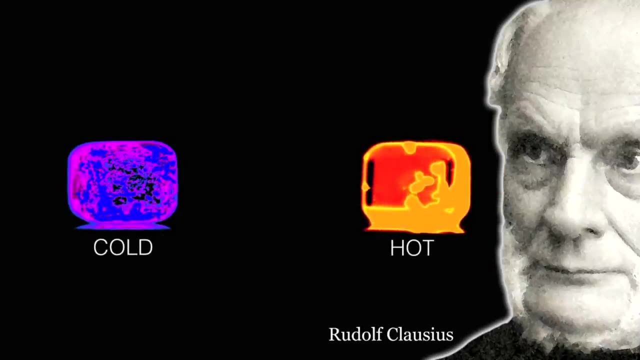 entropy and disorder was invented and they were very kind of operational definitions of it. so there were two classical statements of the second law of thermodynamics. the first is one due to a guy called Clausius who said that heat won't travel from our cold body to a hot body, and that's sort of trivially. 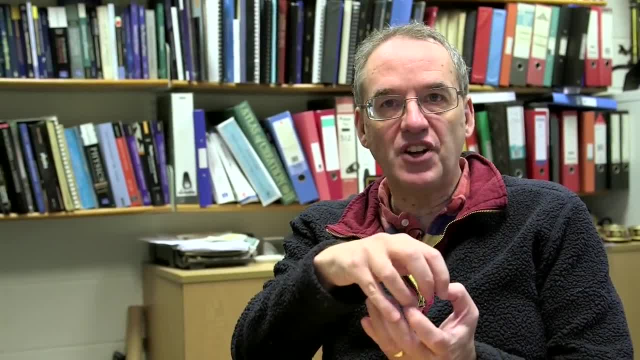 known, if you've just got a hot body and a cold body and you put them in contact with each other, the heat will flow from the hot thing to the cold thing, so they'll end up at the same temperature. they'll meet somewhere in the middle and 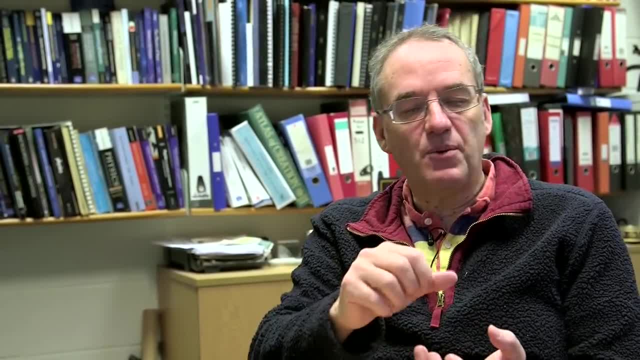 so that's the first law of thermodynamics and the second law of thermodynamics is the third law of thermodynamics. so it's kind of obvious if you're just doing, you know, putting things in contact with each other. but his statement is stronger than that which is: there is nothing you can do to make heat flow from a cold body to. 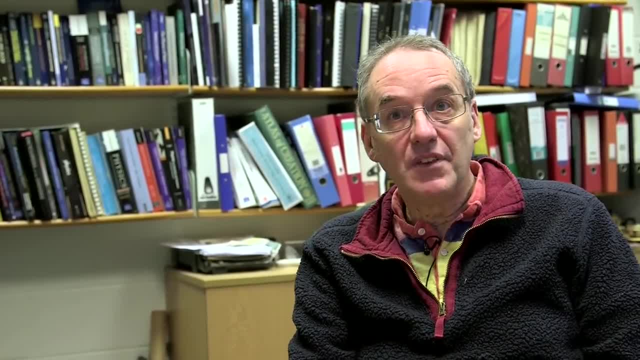 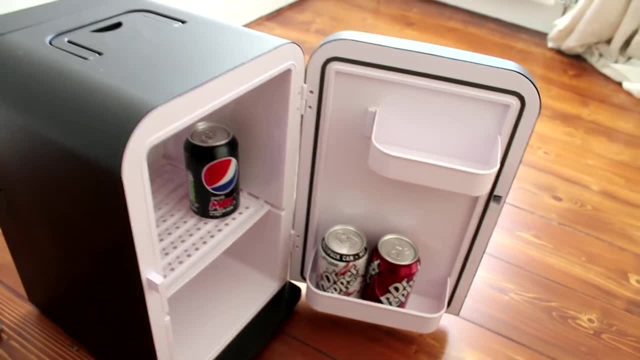 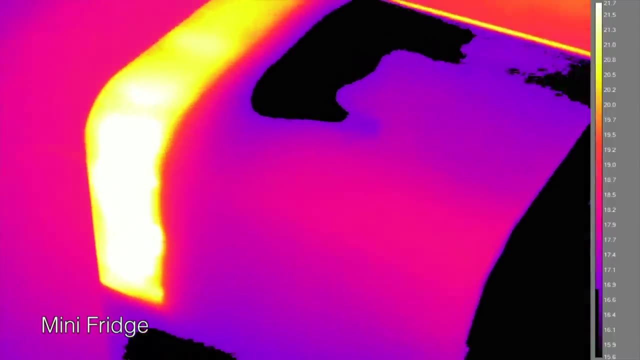 a hot body without putting some work in. so if you're prepared to inject some energy, you can make hot things colder and cold things hotter. and so you know, a fridge is an example where you pump heat out of something which is already cold and add it to the air which is warmer. so fridges, you know, in some sense they 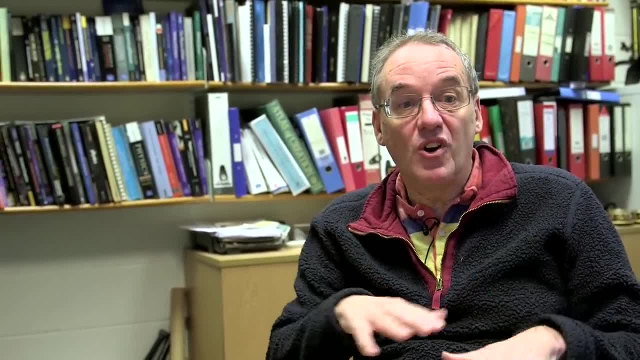 violate the principle of thermodynamics. and so it's kind of obvious, if you're going to violate the purest view of this view of this law, that you can't get heat to travel from something cold to something hot. but the get out is, but you're putting work. 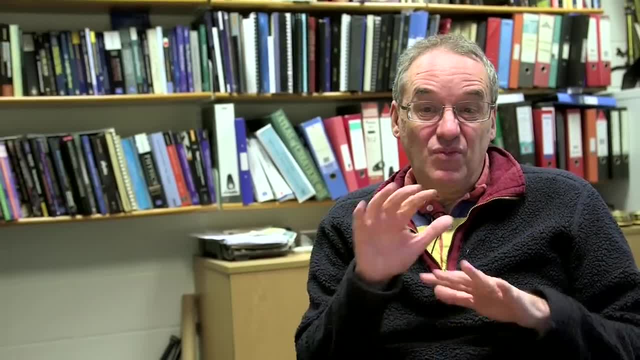 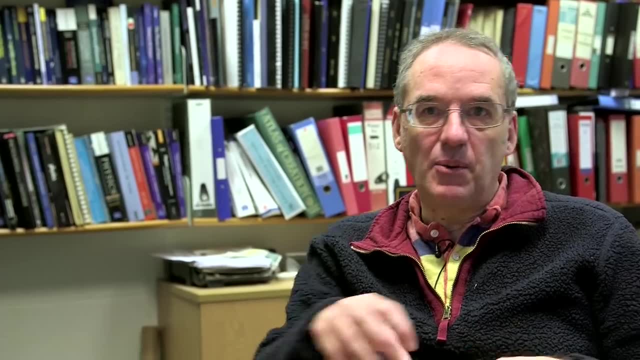 in so you're allowed to do it. so if you've just got an isolated system, you can't do it. it's a one-way street and there's no way around. it is the important point that, no, no matter how clever a machine you come up with, you can never make it so it will extract the heat from the 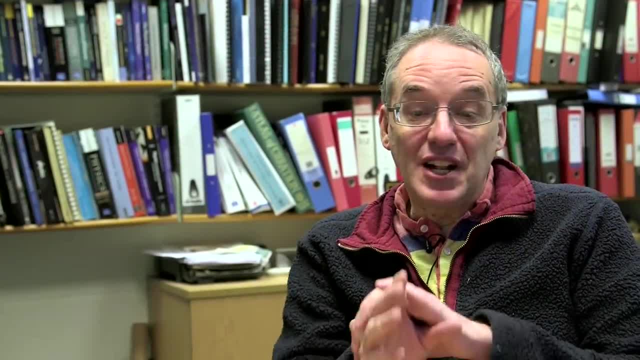 colder thing and add it to the hotter thing without having to put some work in along the way. so that was Klaus's statement, and then this, uh, the other statement, and that's that's. in some sense that's a sort of physicist statement, because that's about 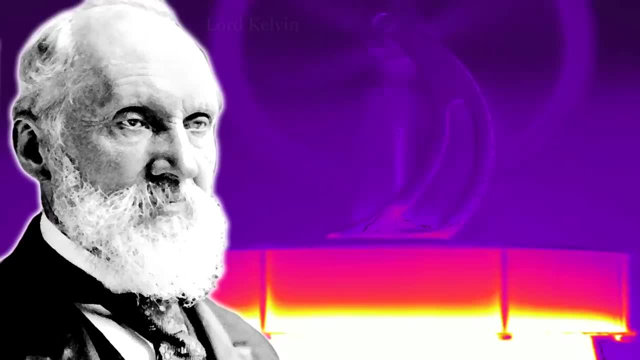 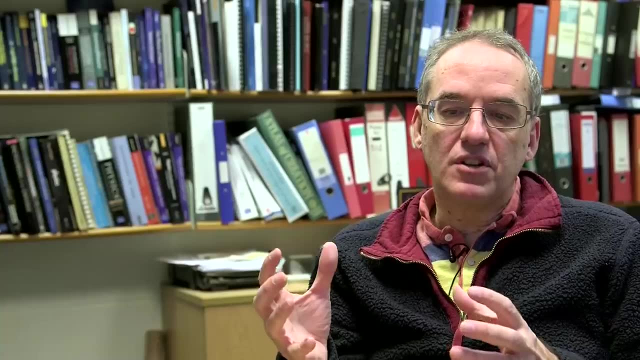 you know heat flow and observations of what happens when you put bodies in contact with each other, the. the second version of this is due to Lord Kelvin, and Kelvin's statement is more of an engineer's statement. this comes back to this fact that there are these two sorts of energy. 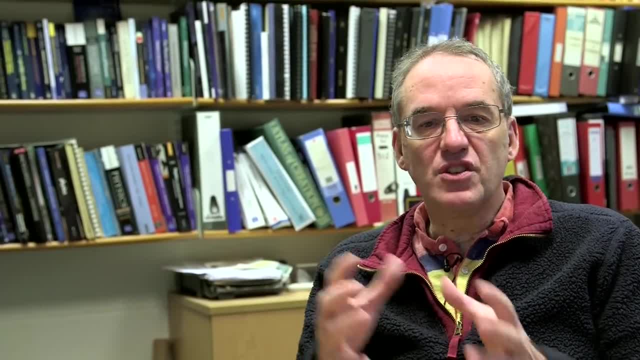 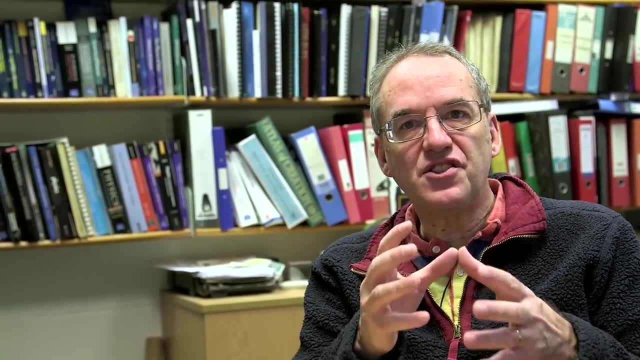 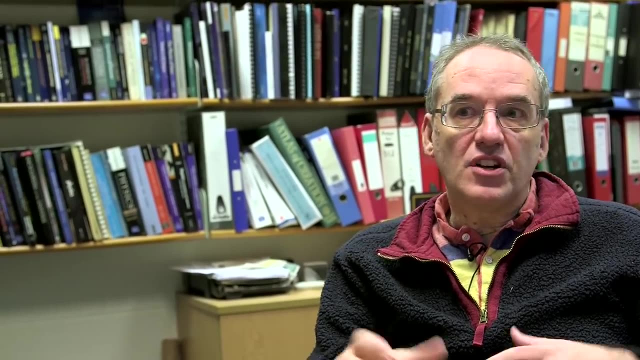 there's kind of useful energy that you can do work with and there's useless energy, heat that you can't really do work with directly, and Kelvin's statement basically says that you can't turn heat directly into work. you can't just take heat and turn it into into useful energy. now, of course again. 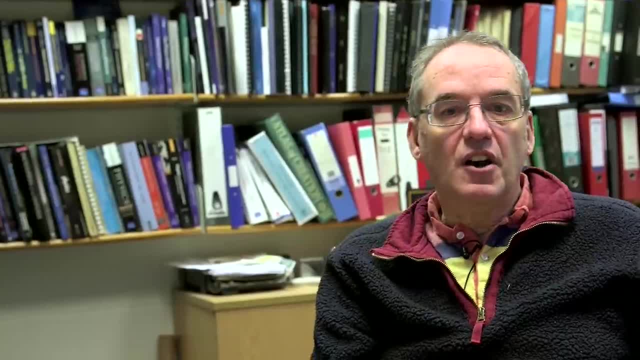 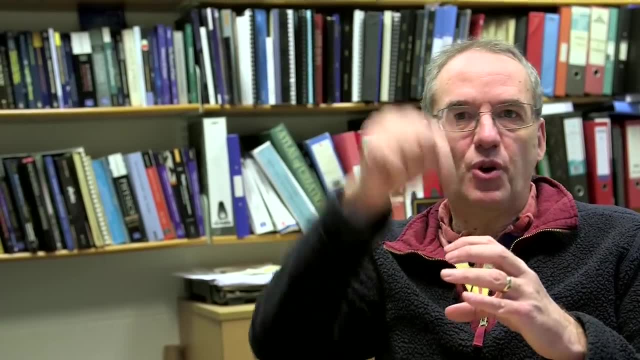 if you do this, a steam engine, for example, takes heat and turns it into work, but in order to do that, you have to have waste heat left over. so his statement is that you can't again have a kind of sealed box where you just put heat in at the top and the only thing that comes out is work. 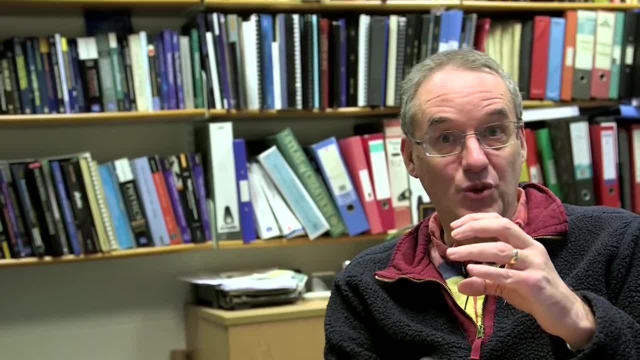 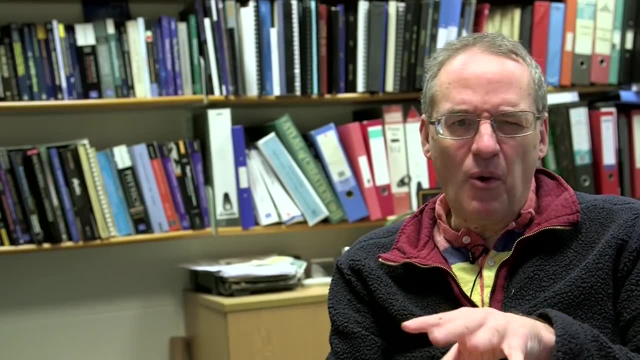 you're always going to have to have heat going in, work coming out, but then some waste heat coming out as well. there is a fundamental limit as to how little the amount of waste heat there is that you can get out of it, and you can figure out what that limit is, but but it's always a finite amount. 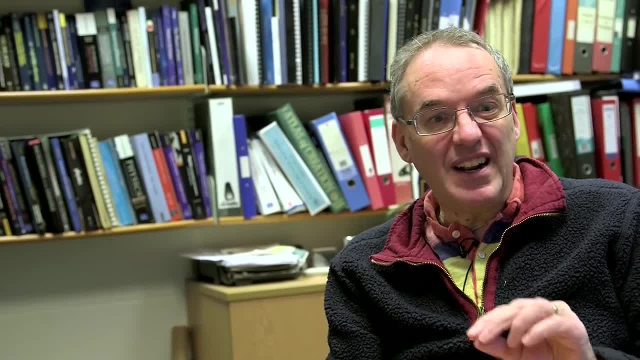 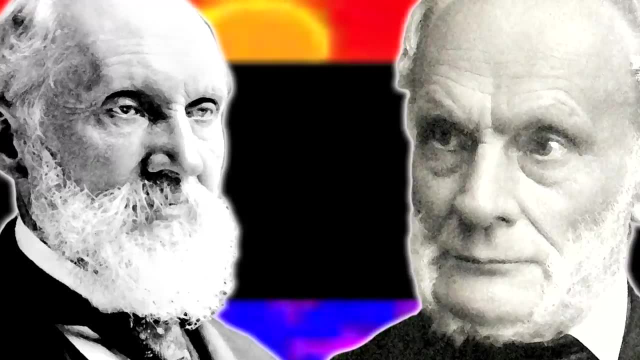 you can't, you can never reduce that to some you know. you know, completely infinitesimal or zero level. those two things sound like completely different statements. right, they're talking about completely different things, but it turns out they're exactly equivalent to one another, and I can show you, if you like. so the way we're going to do this is by saying: if one of these 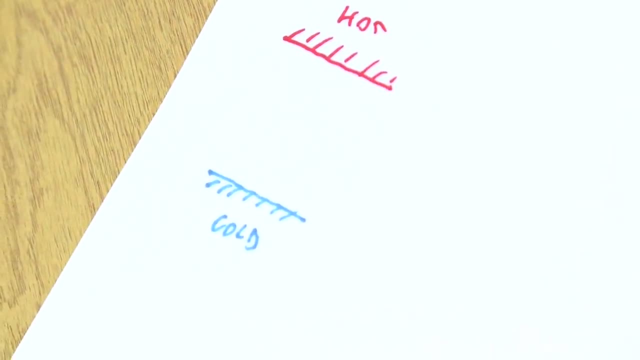 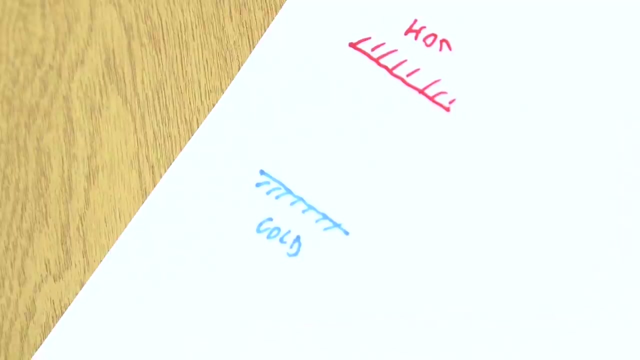 versions of the second law isn't true, then the other one isn't true either. so let's assume let's violate Clausius's statement of the second law, which basically says you can't get heat to flow from the cold body to the hot body. so let's assume we have a magic fridge which violates that law by. 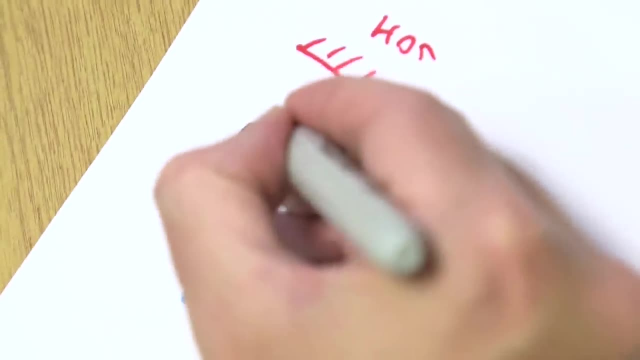 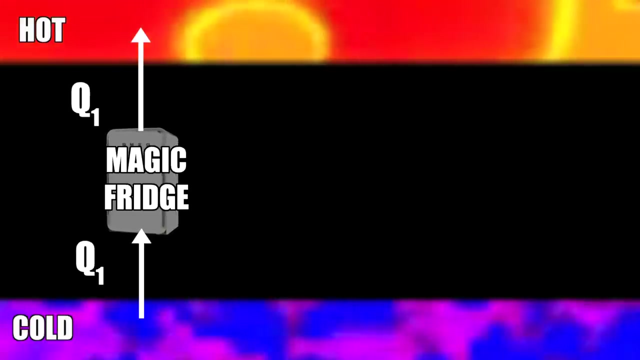 actually allowing us to suck energy out of the cold body, put it into the hot body without actually having to plug the fridge into the mains. okay, and then on the over here, I'm going to just have a, a, an engine like a steam engine or something that which doesn't violate any of the laws at all, and I'm going to take an amount. 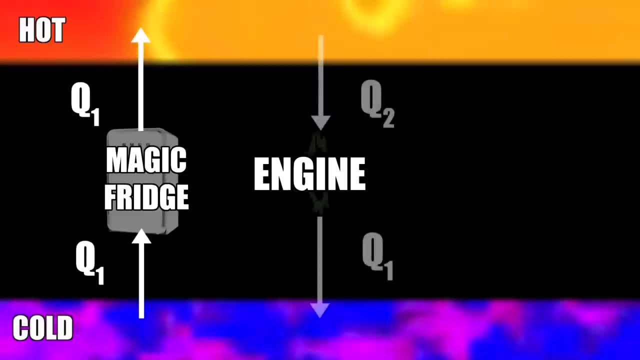 of energy out of this hot body- you too. and because this isn't breaking any laws, there has to be some waste heat from it, so we'll set it up so that amount of waste heat is actually equal to Q1, keeping Lord Kelvin happy. so, yes, exactly, that's not violating any of the laws and we're going to. 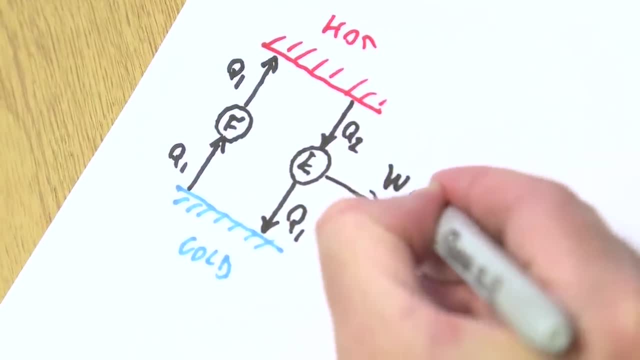 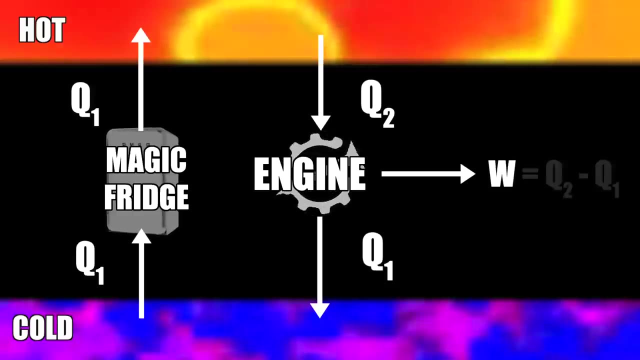 get some work out of this, which is just the difference between those two. this is the first law, again that says that you have to conserve energy overall. so if we've got Q2 flowing in and then the amount of work we get out of there is just the difference between the two. now, the neat part here is that what we've 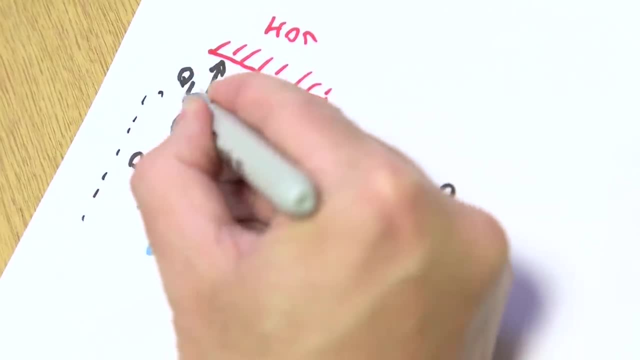 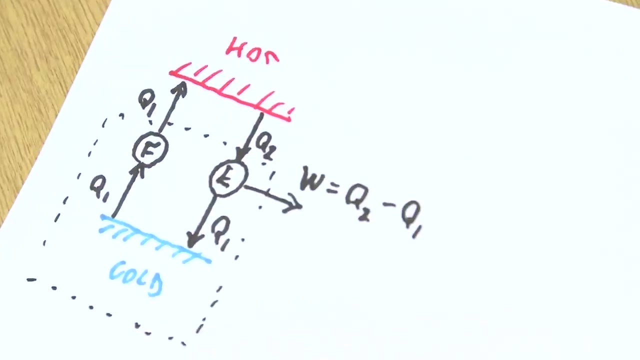 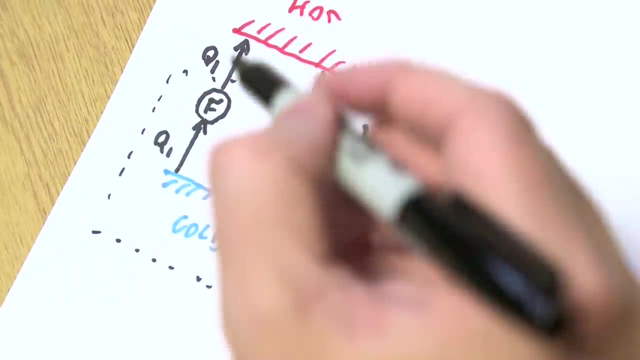 managed effectively to do. if I just draw a box around this little lot here and say that's just going to be, I'm going to stick all that on in a box and I'm not going to care what's inside that box. and what that box is actually doing is it's. 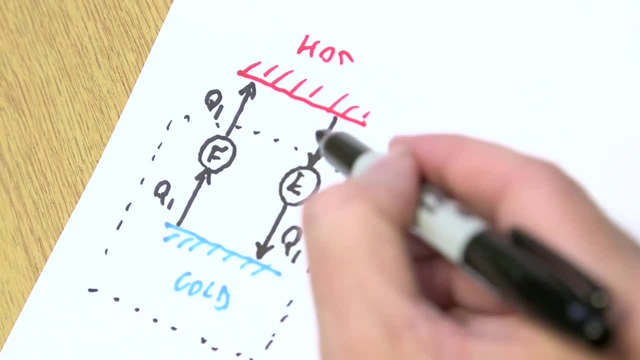 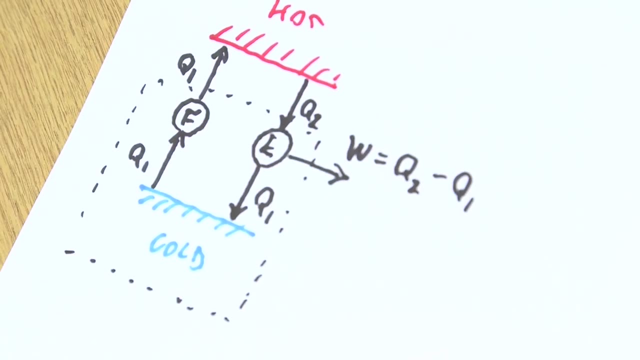 taking an amount of energy. well, how much energy is coming in? it's taking heat out of this body and it's taking an amount. well, there's Q2 flowing out and Q1 flowing back in. so the amount of energy that's coming out of this hot body is Q2 minus Q1 and this box, then the only thing that's coming out. 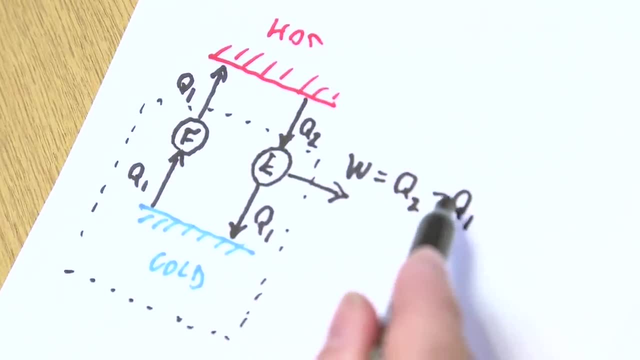 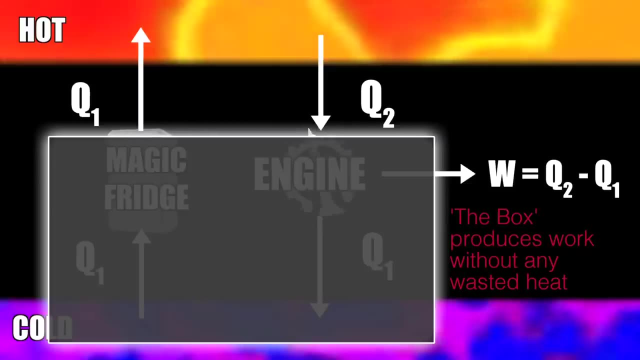 of it is work Q2 minus Q1. so this now violates Kelvin's version of the second law, because actually we've what we've. all we've done in this process is we've taken an amount of heat out of this hot body and turned it directly into work, and Kelvin's statement of the law says you can't. 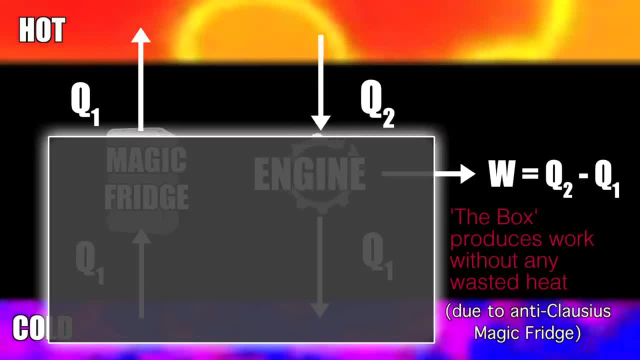 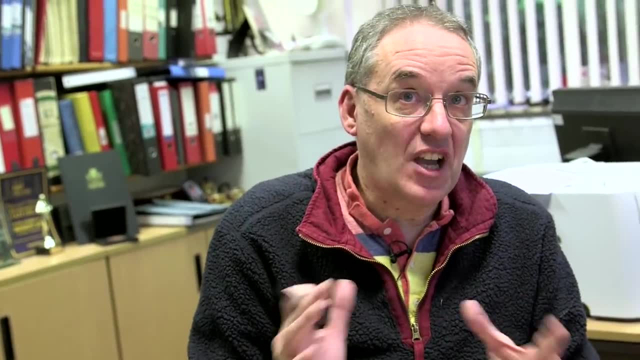 do that, Professor, that shouldn't be a surprise, because we built the box by breaking the rules. we just broke Clausius's wording of the rules exactly. but what we're trying to show is that those two statements of the second law are the same as each other. they're really stating the 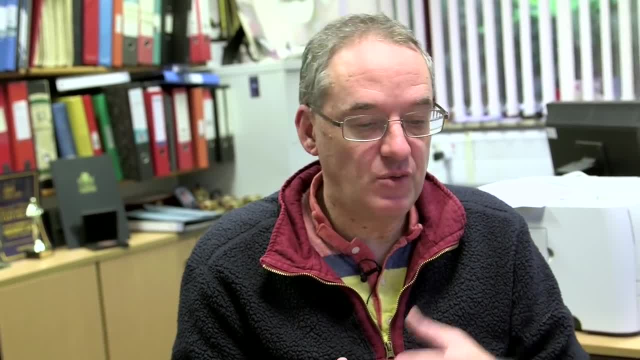 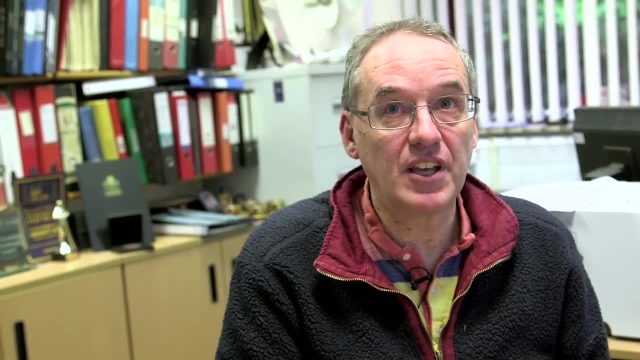 same law and so, indeed, if they are the same law, you'd expect if you broke one version of the law, you'd break the other version of the laws as well. but if they're actually different laws or they're stating different things, then that wouldn't necessarily be the case, but that's kind of. 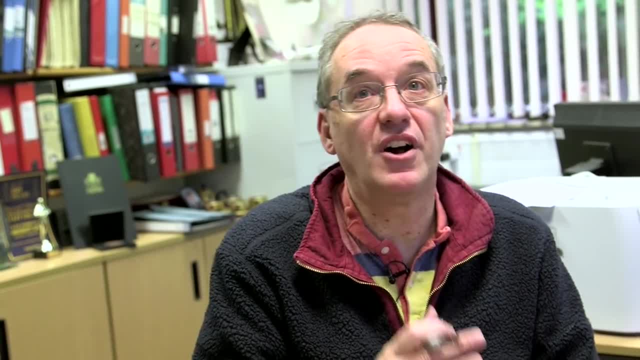 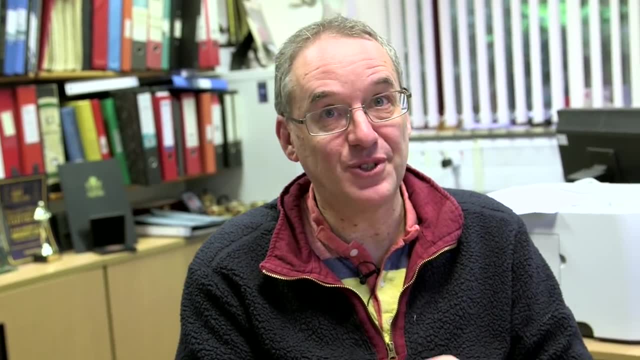 halfway there. that shows that if we violate Clausius's version then we're violating Kelvin's version. to really show their equivalent, we've also got to show if we violate Kelvin's version, we're also violating Clausius's version. okay, okay. so Kelvin's version of the law says that you can't. 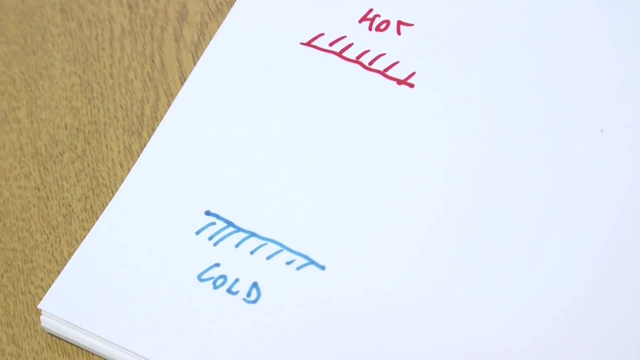 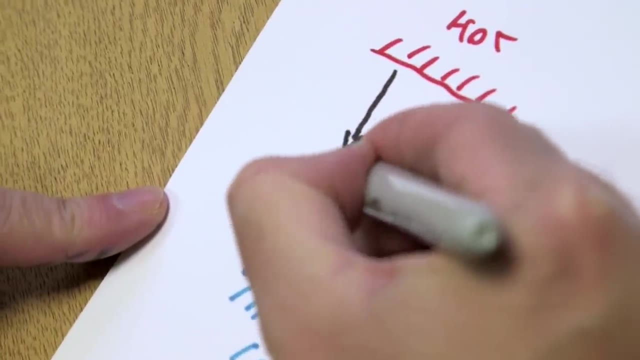 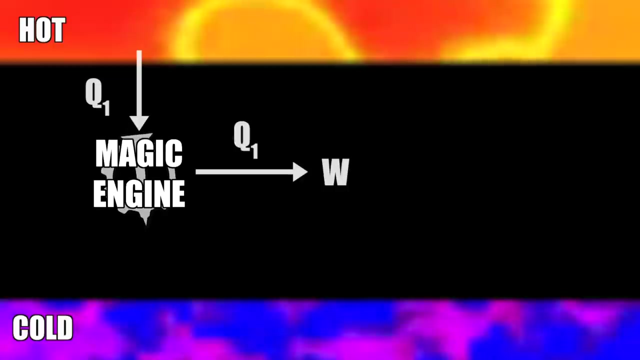 just turn energy into work. so you can't just take heat and turn it directly into work. that has to be a byproduct. so let's violate that by coming up with a magical engine which directly turns energy, turns heat into work, an engine which, yeah, which does nothing but take this useless energy heat. 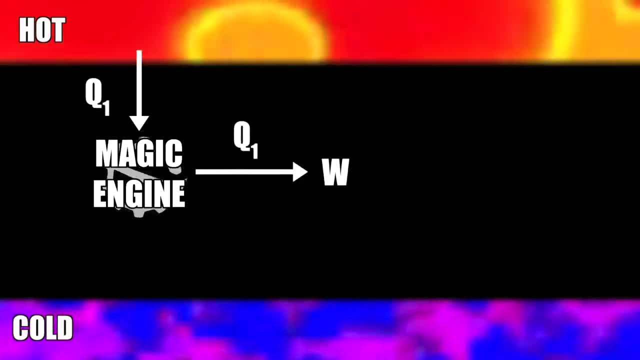 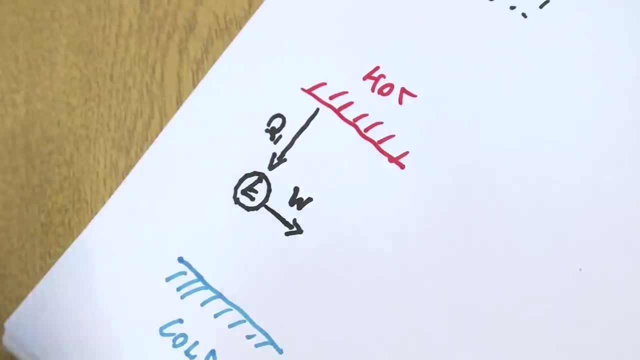 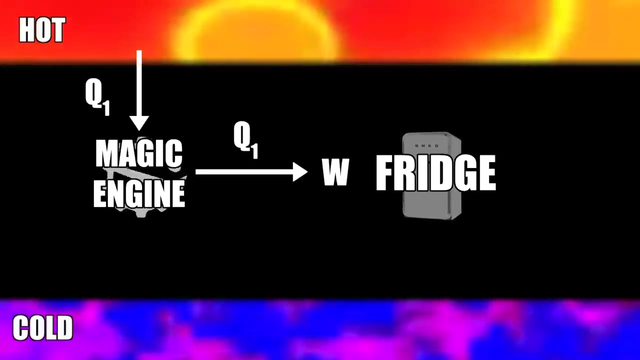 and turn it directly into useful energy work. infinitely efficient steam engine, so a real steam engine. there'd be waste heat coming out the bottom, but we're violating Kelvin's law here so we don't have to do that, okay, okay, and then we're going to take that work and we're going to use it to power a fridge. okay, and that fridge will, because this is. 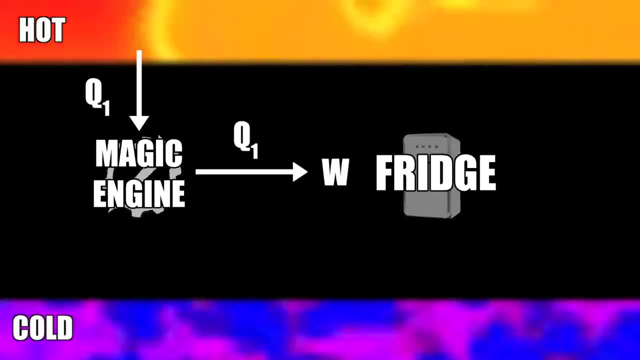 now a proper fridge. it's not violating Clausius's law or anything. we can get it to work. so we've plugged it into the mains and we can actually use it to suck energy Q2 out so we can figure out how much heat's going to come out the other end. 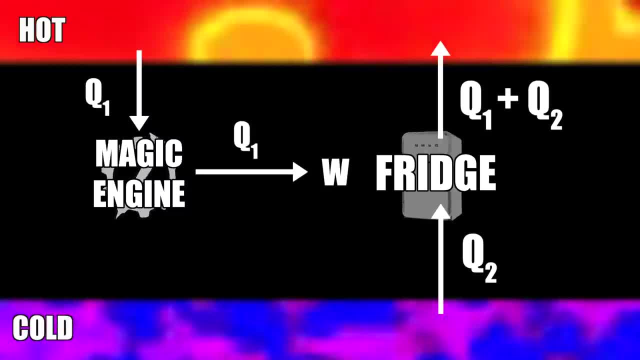 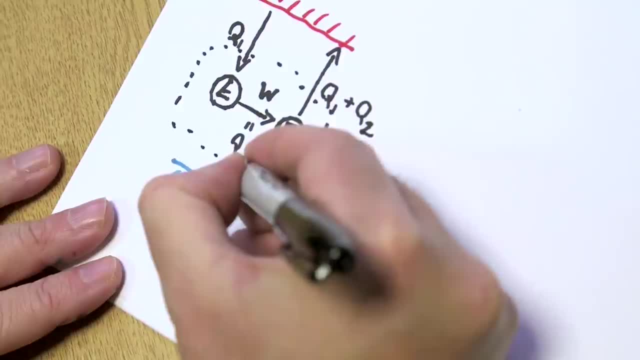 it's just going to be the two lots of energy going in as Q1 and Q2. so now, if we just put a box around all this lot and say this is, this is now my magic machine, and I don't really want to look inside the box, I just want to know what it's doing, what's happening. it's sucking an amount of.